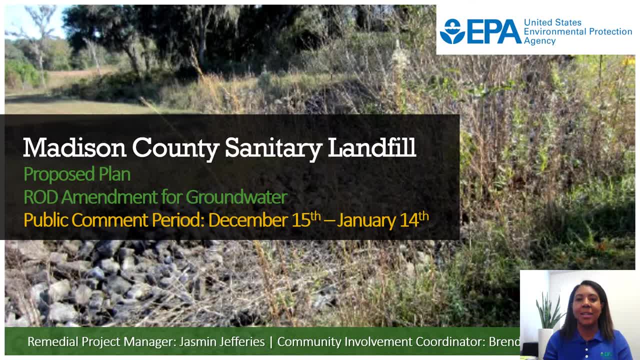 presented in the feasibility study and summarize in the proposed plan. These documents can be found on the site webpage at wwwepagov. forward slash Superfund. forward slash Madison hyphen, county, hyphen sanitary hyphen landfill. The public comment period will be open from: 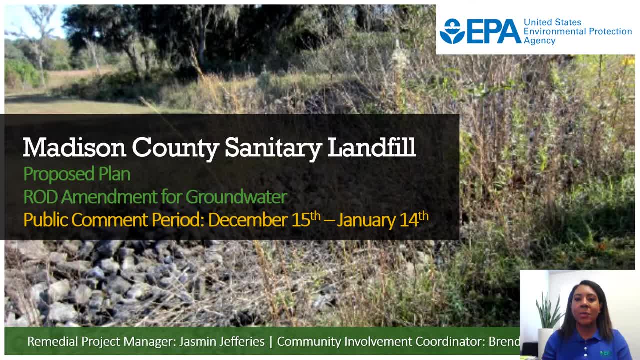 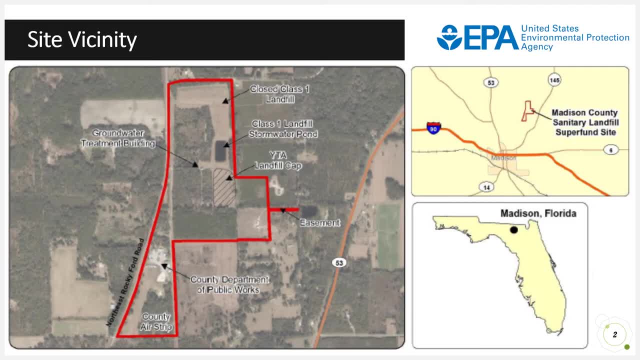 today, Wednesday December 15th, through Friday January 14th. More details on how to submit your comments and or questions will be available. The Madison County Sanitary Landfill site is in a rural area in Madison County, approximately 2 miles northeast of the city of Madison Florida. The total site occupies 90 acres. 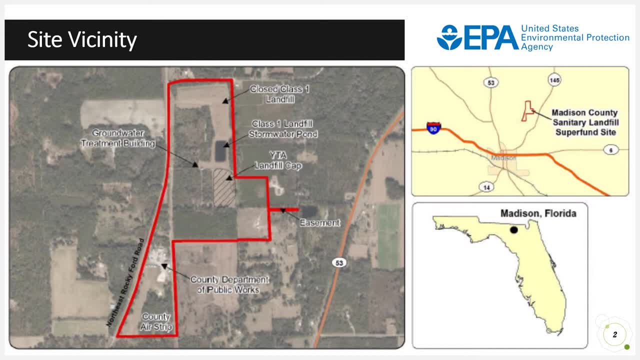 The Captain Fence Former Landfill, also referred to as the Yard Trash Area or YTA, is approximately 9 acres. Domestic waste, as well as local industrial waste, was disposed of in the YTA from 1970 to 1980. Disposed of in the 1970s and 1980s. Disposed of in the 1970s and 1980s. Disposed of in the. 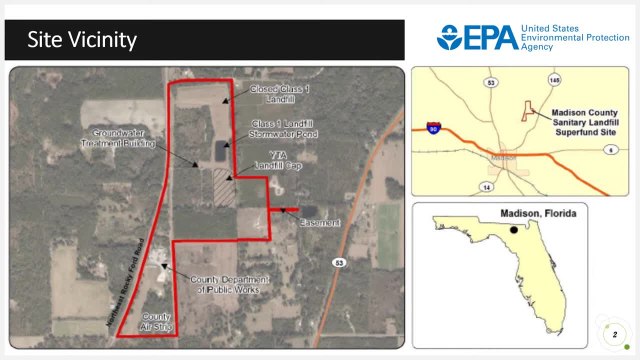 1970s and 1980s. Disposed of in theelp And noise pollution may have implanted in your decontaminated element, often at the rate of upload rate. Disposed operations result in the contamination of soil and groundwater with chlorinated. 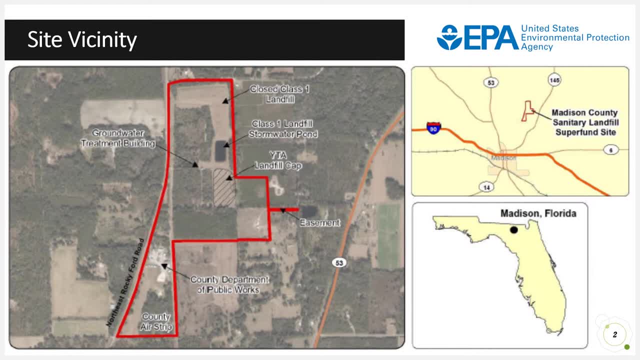 volatile organic compounds. The only residence within the vicinity of the site is a home located on a hill about 800 feet to the southeast. The county's public water supply comes from wells located in the city which are not impacted by the site. Any city residences are connected to public. 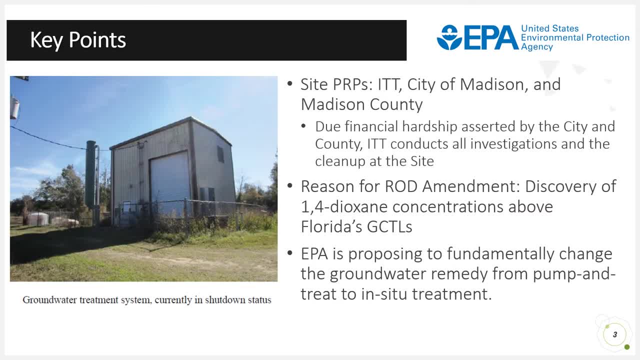 water line supply lines, The site as a potential respondent parties or prior p and p and our private wisdom KIME are itt the city of madison and madison county, due to financial hardship asserted by the city and county itt conducts all investigations and the cleanup at the site. 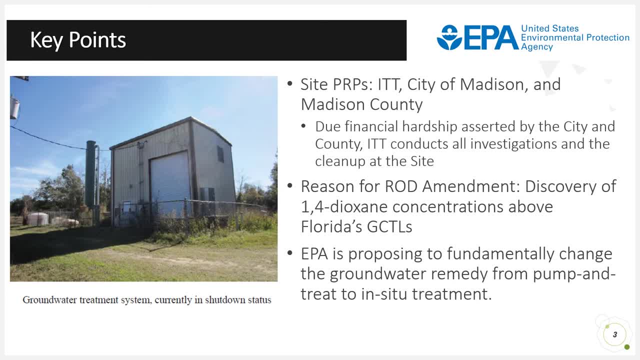 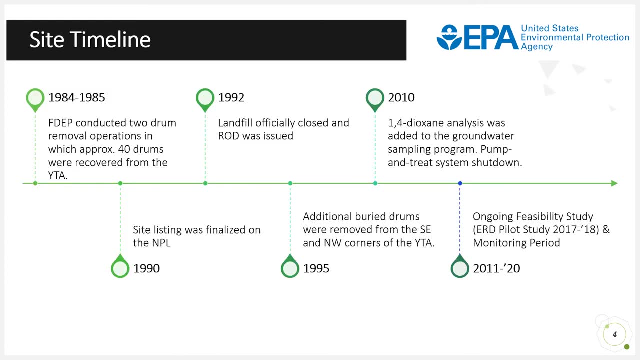 the reason for the rod amendment was the discovery of one for dioxane concentrations above florida's groundwater cleanup target levels. epa is proposing to fundamentally change the groundwater remedy from pump and treat to in-situ treatment. from 1984 to 1985, fdep conducted two drum removal operations. 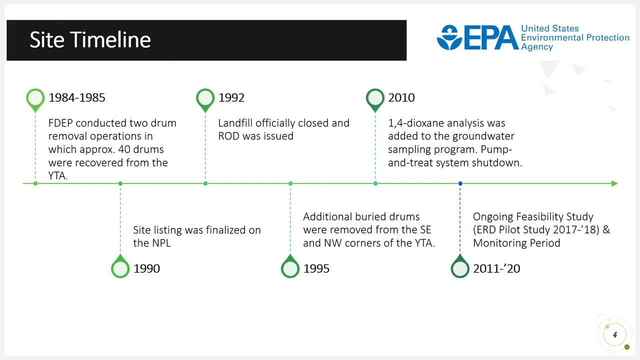 in which approximately 40 drums were recovered from the yta. in 1990 the site listing was finalized on the national priorities list, otherwise known as the npl. in 1992 the landfill was officially closed and a record of decision was issued in 1995. 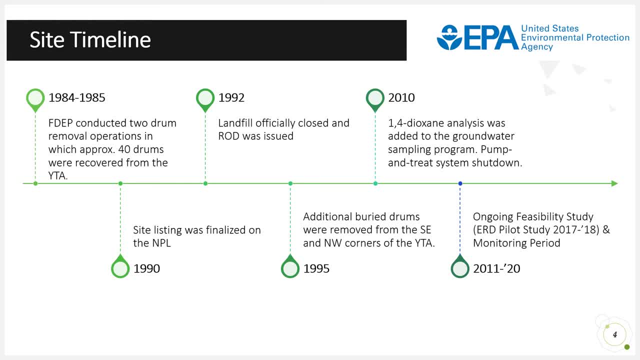 additional buried drums were removed from the southeast and northwest corners of the yta in 2010, one four dioxane analysis was added to the groundwater sampling program. the pump and treat system was shut down due to concentrations detected in the floridan aquifer above florida's gctls. in 2011 to 2020, an ongoing feasibility study took. 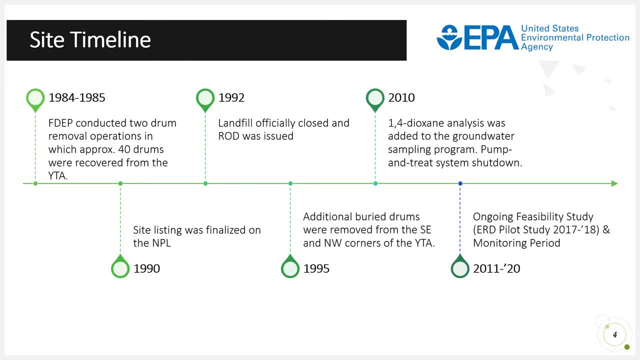 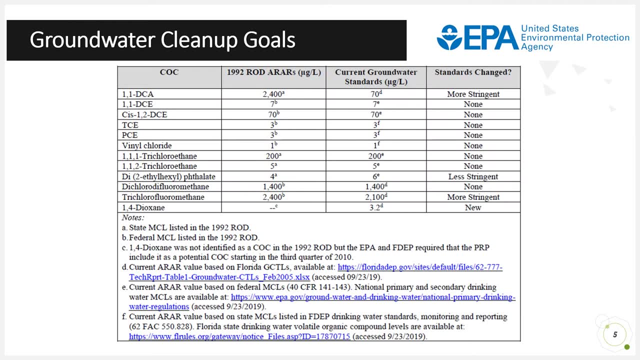 place, which used enhanced induct, enhanced reductive dechlorination. all of the chlorinated volatiles were removed from the yta. the first monitoring being conducted was conducted here with the help of a group of organic compounds, and uhhere's an example of what the 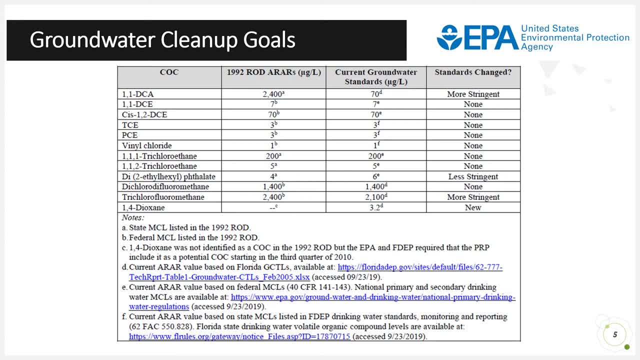 conduct was like, say, no임alardy, for example. the number of organic compounds listed in the left-hand column are contaminants of concern at the site, with the exception of one for dioxane, which will be added as a coc in the rod amendment. the semi-annual monitoring reports review trends for eight wells that have 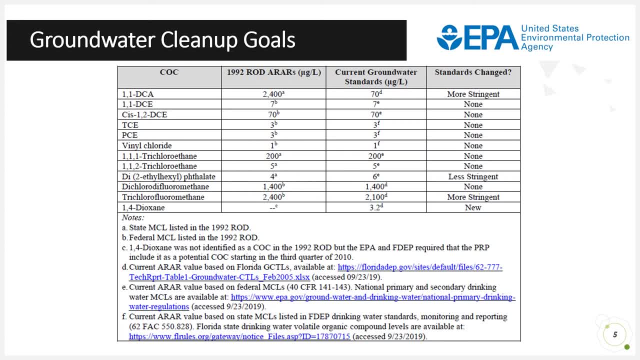 historical long-term data for cvocs southeast of the yta in the east portion of the yta and the northwest portion of the yta. five chloroethylene or TCE trend and corresponding trends of the TCE degradation products- cis-1,2-DCE. 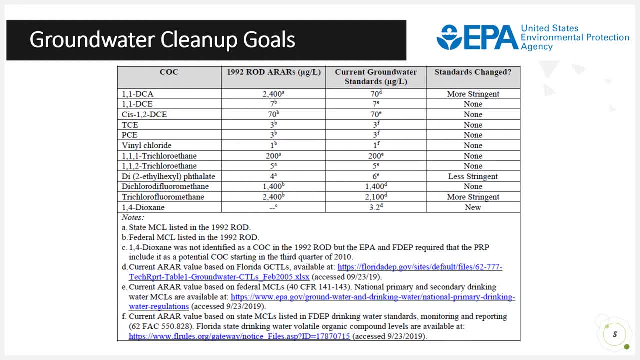 and or vinyl chloride in the southeast YTA and the east YTA, as well as the northwest YTA. Two of the wells show an overall decreasing trend for all CVOCs in the eastern portion of the YTA and one well shows an increasing trend for all CVOCs. 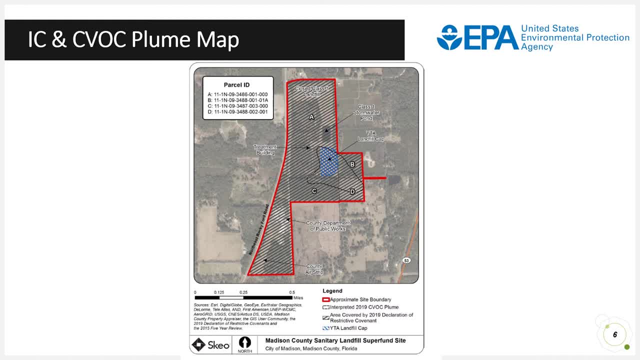 Pictured is the institutional controls map and CVOC plume. Primary source of contamination is the former Madison County landfill yard trash area which is outlined in blue. The primary release mechanism were contaminants and buried drums leaching into soil and groundwater. The site is under water. 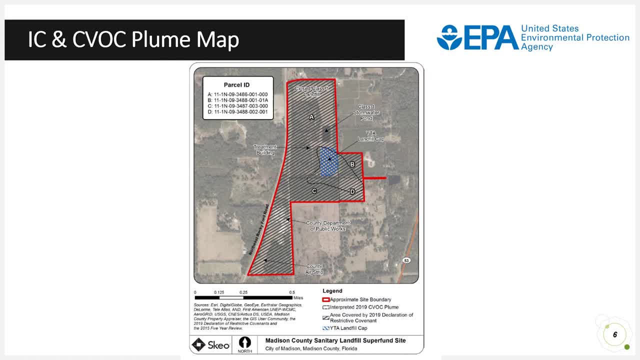 There are one operable unit site-wide OU-1,, and it addresses soil and groundwater. Soil contaminants have been capped and fenced and the remedy is operating as anticipated. The Rodd Amendment is to address groundwater restoration. only Three remediation alternatives for groundwater are being considered for this site. 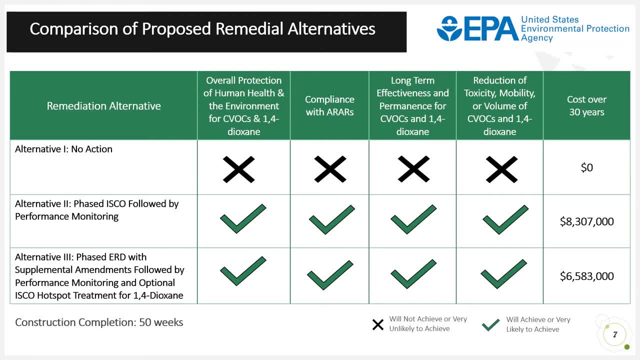 Alternative 1,, as the name suggests, would require no action. It would not be protected, It would not be effective, of human health and the environment. It would not comply with applicable or relevant and appropriate requirements, otherwise known as ARRs, It would not be effective in the long term and it would not treat the COCs at the site. 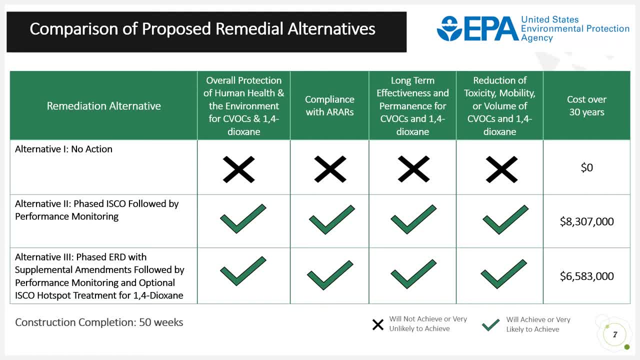 The cost of a no action remedy at the site would be $0.. In every feasibility study, a no action alternative is developed as a baseline for comparative analysis purposes. A no action remedy is not appropriate for the Madison County Sanitary Area. A no action remedy is not appropriate for the Madison County Sanitary Area. 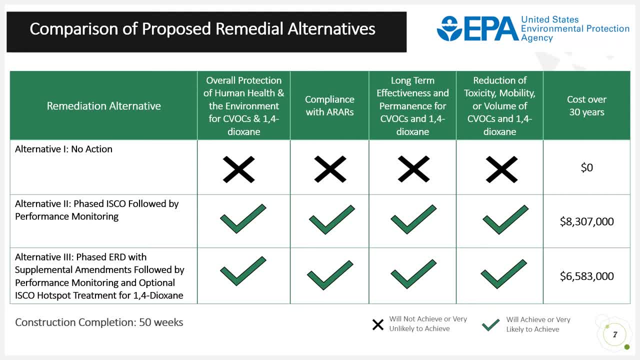 A no action remedy is not appropriate for the Madison County Sanitary Area. So why must we select a reactor site without intimacy? Alternative 2 consists of phase in situ chemical oxidation followed by performance monitoring. This process consists of oxidation reduction, chemical reactions involving the 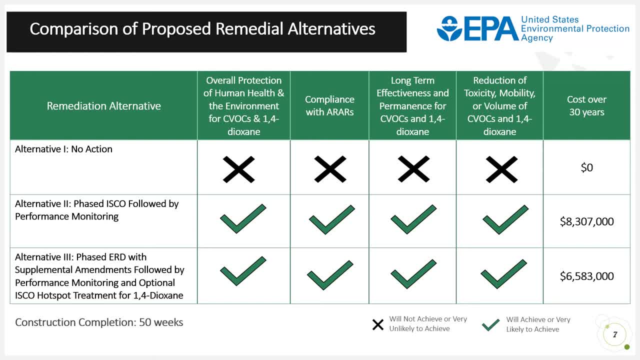 transfer of electrons from one compound to another, thereby making the hazardous compound to be less toxic. Alternative 2 would be protective of human health and the environment. It would apply with an ARR, RARs, it would be long-term effective and it would reduce the concentrations of COCs. 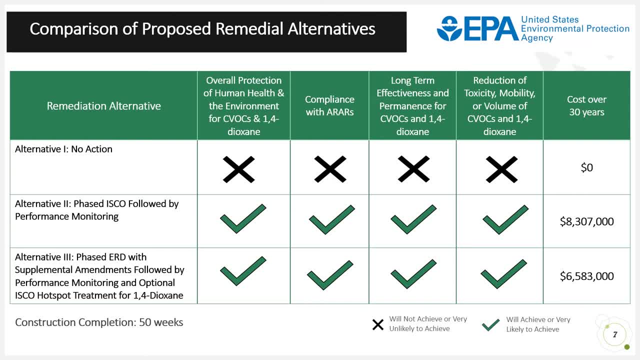 The cost for Alternative 2 would be $8,307,000.. Lastly, Alternative 3, the preferred alternative is phased enhanced reductive dechlorination with supplemental amendment, followed by performance monitoring and optional in-situ chemical oxidation. hotspot treatment for 1,4-dioxane. 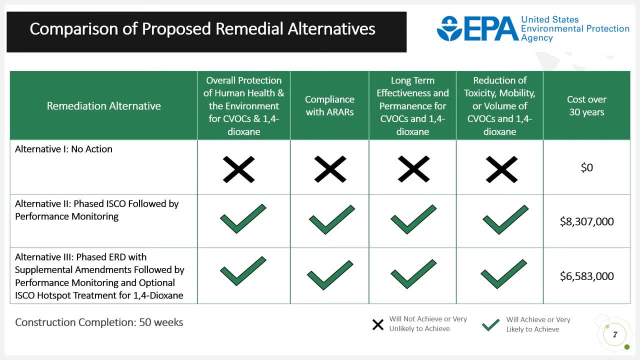 and vinyl chloride if needed. The ERD process is used to accelerate the national biodegradation process by providing a carbon source, nutrients and electron donors to enhance the rapid conversion of CVOC contaminants to non-toxic end products. Emulsified vegetable oil, or EVO, is a common 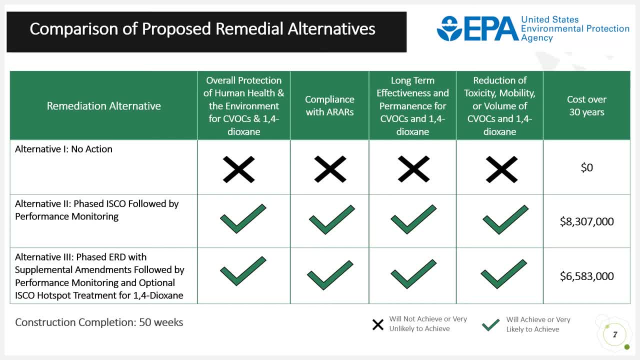 supplemental electron donor used to enhance the natural biodegradation reductive dechlorination process and is what would be the most effective way to reduce CO2 emissions. Alternative 3 would be used at the site if selected Supplemental amendments would be used in conjunction with the vegetable oil to induce anaerobic 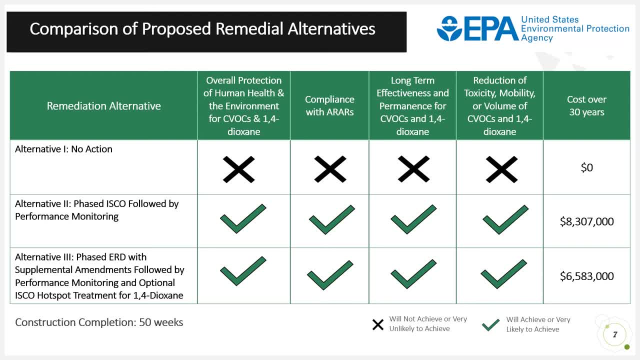 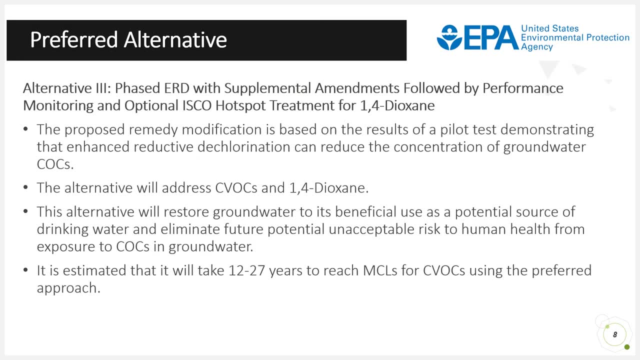 conditions for the bacteria. The cost for Alternative 3 is $6,583,000.. Construction completion for Alternative 2 and 3 would be around 50 weeks. Alternative 3 phased enhanced reductive dechlorination with supplemental amendments, followed by performance monitoring and optional 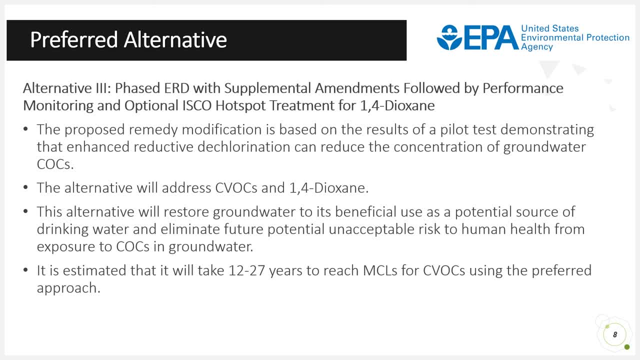 in situ chemical oxidation hotspot treatment for 1,4-Dioxane is the preferred alternative. The proposed remedy modification is based on the results of a pilot test demonstrating that enhanced reductive dechlorination can reduce the concentration of groundwater COCs. The alternative will address chlorinated volatile organic compounds and 1,4-Dioxane. 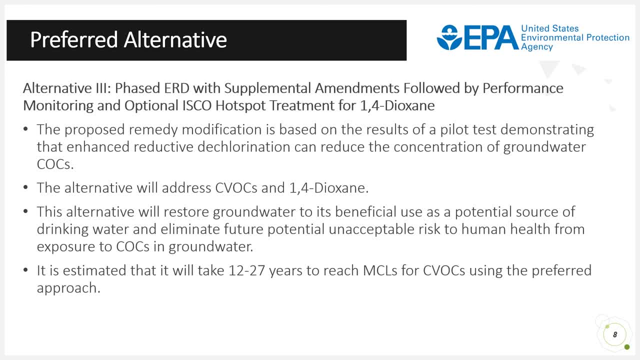 This alternative will restore groundwater to its beneficial use as a potential source of drinking water and eliminate future potential unacceptable risks to human health from exposure to COCs in the groundwater. It is estimated that it will take 12-27 years to reach MCLs for CVOCs using the preferred 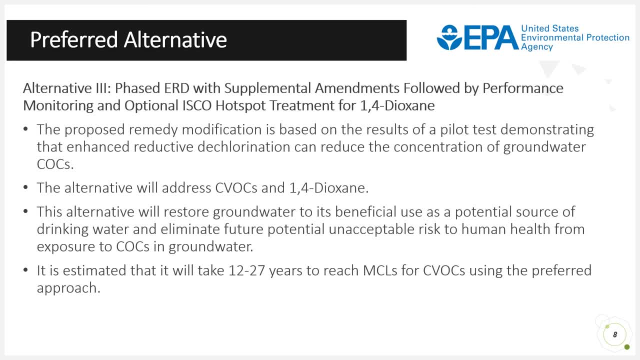 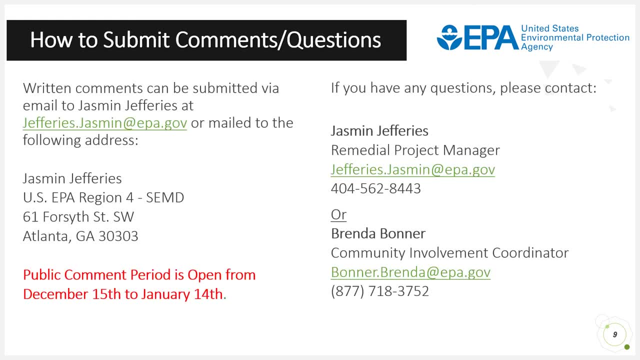 approach. However, this estimated time frame will be refined during the remedial design process. Thank you. Written comments can be submitted via email to myself, Jasmine Jeffries, at jeffriesjasmin at epagov, or mailed to the following address: US EPA, Region 4, SEMD 61 Forsyth Street, Southwest. 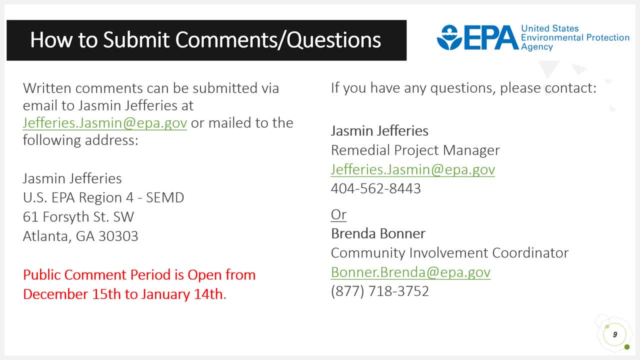 Atlanta, Georgia, 30303.. The public comment period again is open from December 15th to January 14th. If you have any questions, please contact us. Thank you, You can still contact me by email or phone at 404-562-8443. 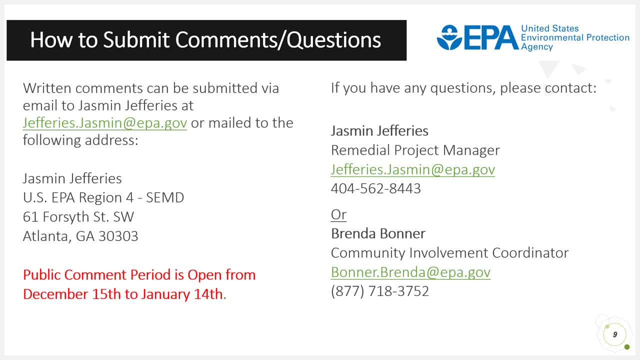 You can also contact Brenda Bonner, Community Involvement Coordinator. Brenda can be reached at Bonnerbrendaepagov or at 877-718-3752.. Thank you again for tuning in to this presentation and please reach out to me if you have questions. Thank you.